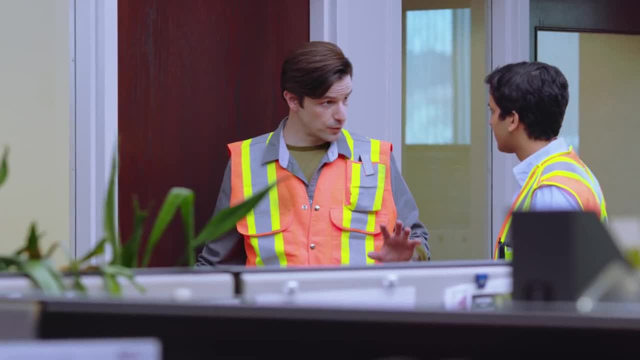 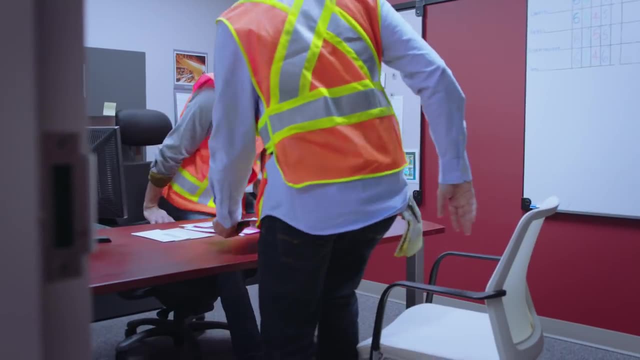 we need to complete a preliminary investigation report, And we need to do it within 48 hours. Then we need to complete an interim corrective action report That'll show what steps we took in the short term to make the area or job safe. Okay, but what exactly do I put in these reports? 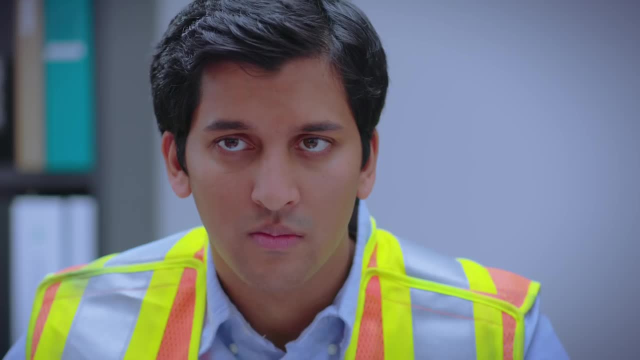 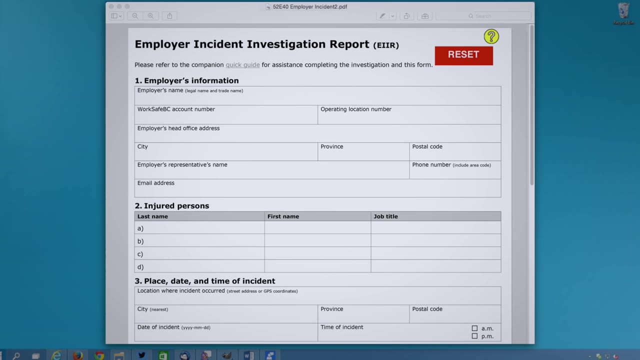 Let's go to the WorkSafeBC website. They have a report template that makes it all pretty easy. Here it is. Now there's a guide on how to fill it out. Most of the information is pretty basic, Like date of the incident, name of the injured worker. 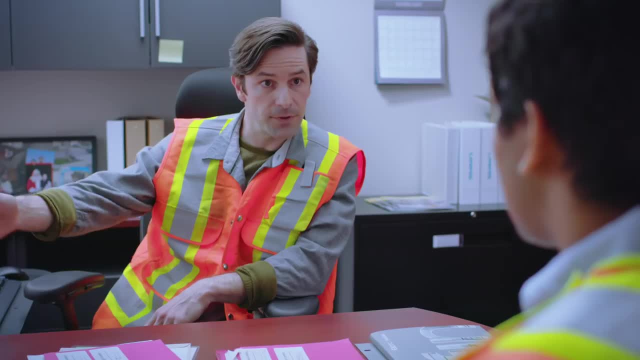 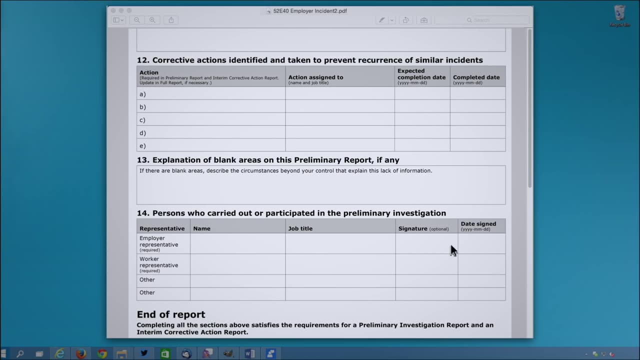 a description of what happened, and so on. Now, if you fill out the form, you'll have addressed all the requirements of the investigation. For the interim corrective action report, you just have to document what you've already done or will do while the full investigation is in progress. 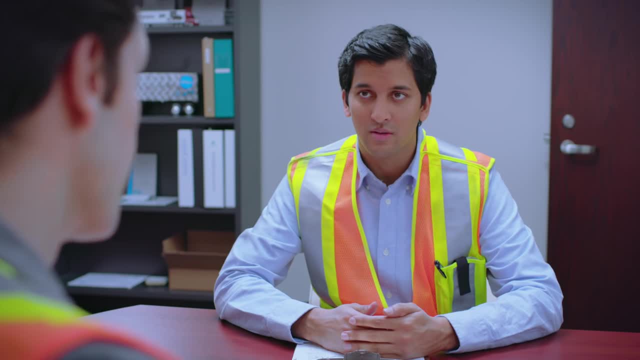 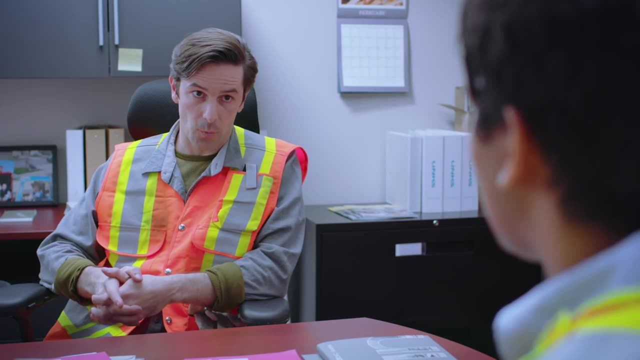 Okay, That's it Not quite. That deals with the immediate issues, But to finish the investigation report, we need to figure out exactly how and why the oil ended up on the walkway. Okay, Well, I've done some work on this. 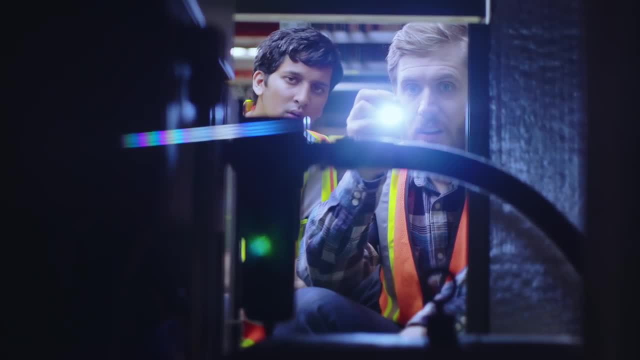 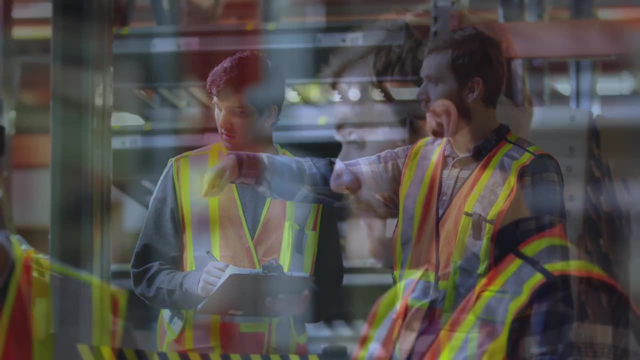 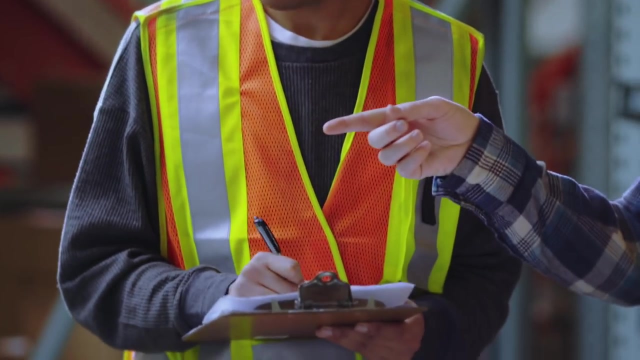 Rich from the Joint Health and Safety Committee and I checked it out. Turns out the oil came from an old compressor and it may have been leaking for quite a while. I've asked maintenance to take it out of service and look at it And we're going to examine our maintenance program as part of a more permanent solution. 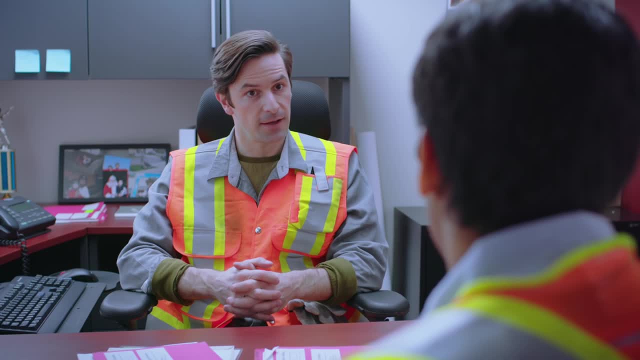 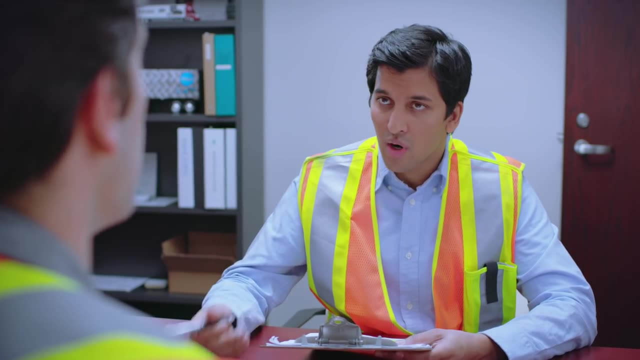 Great. You might find other issues as part of the investigation. We need to make sure this never happens again. That all sounds pretty straightforward and normally I'd wrap it up in a couple of days. The problem is we're doing inventory and I'm really busy. 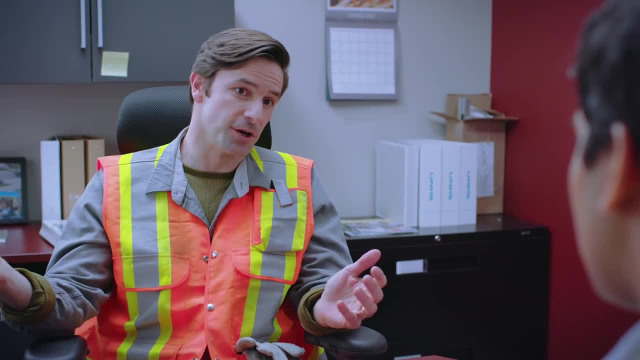 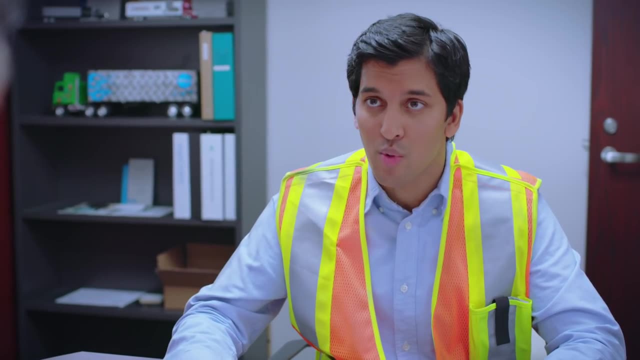 As long as you finish the preliminary investigation within 48 hours, we're good. Then start the full investigation as soon as possible and have it completed in 30 days. Right, and the full corrective action report just needs to be completed as soon as possible after that. 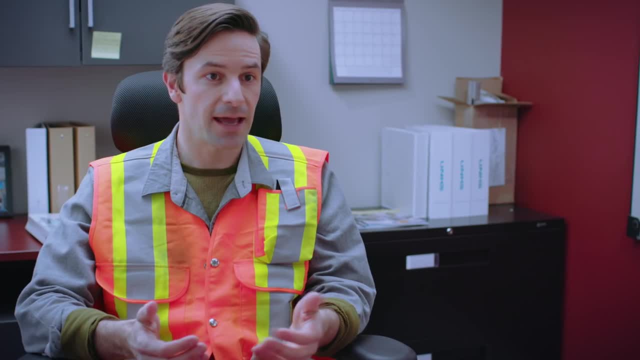 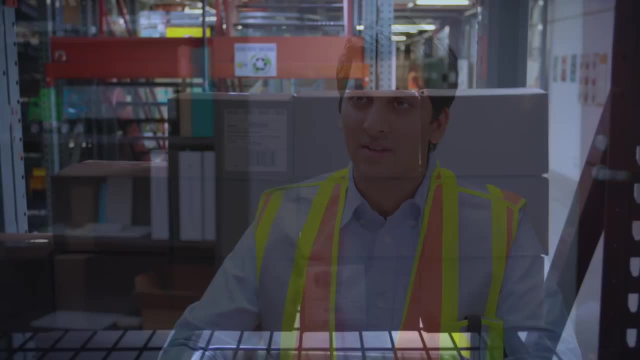 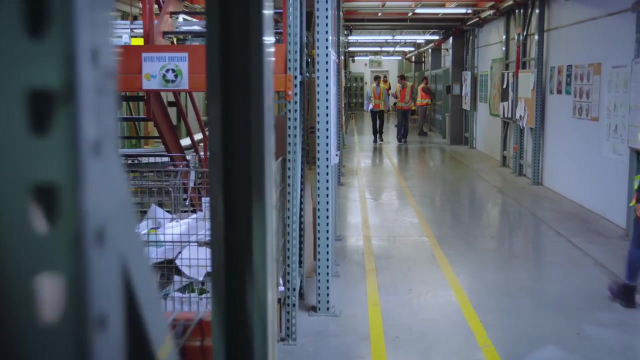 Exactly. And if it turns out the incident is more complicated and we need more time, we can contact a WorkSafeBC officer and ask for an extension. Good to know. So I send all the reports to WorkSafeBC? No, we always send them the full investigation report. 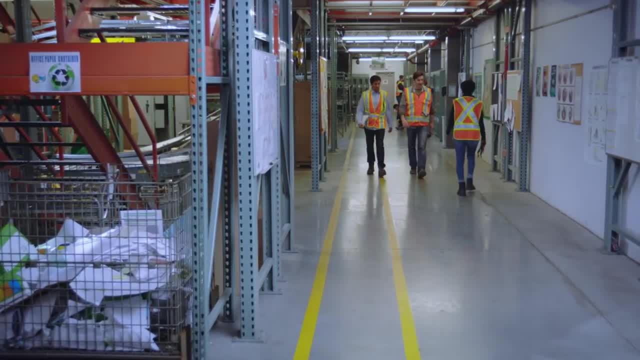 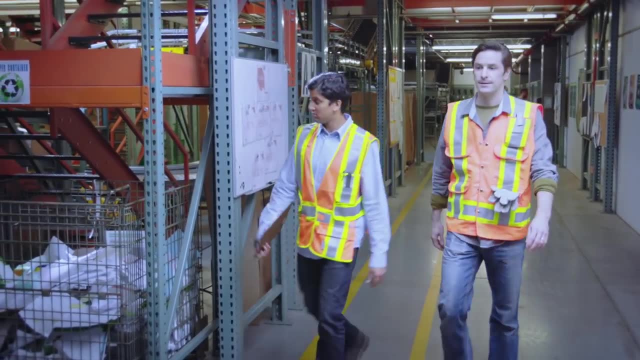 But the other reports, like the preliminary report, only need to be sent if they ask for them, And copies of all the reports need to be sent to our Joint Health and Safety Committee. So that's it. That's it. Give me an update tomorrow on how you're doing and I'll get you an update on Jim's condition. 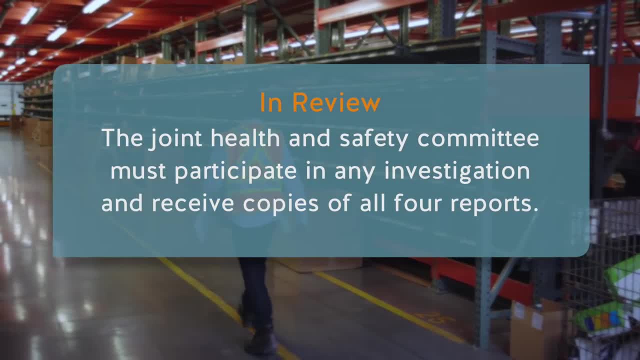 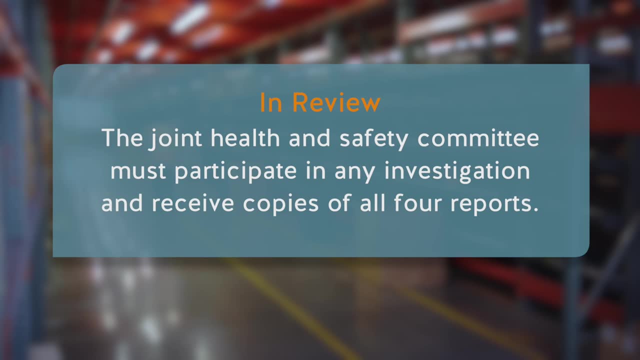 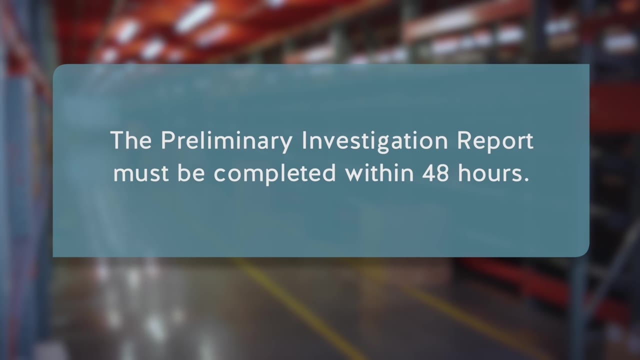 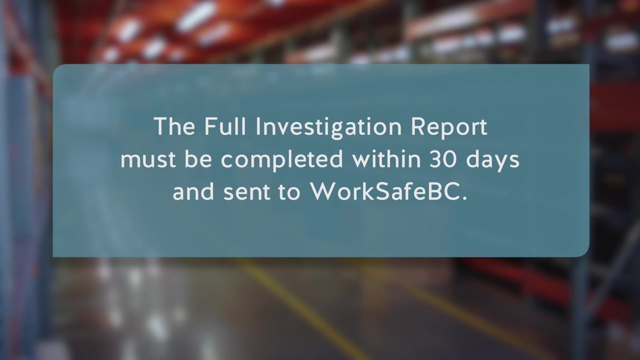 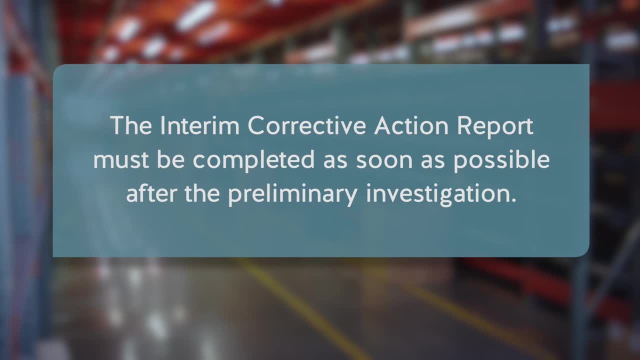 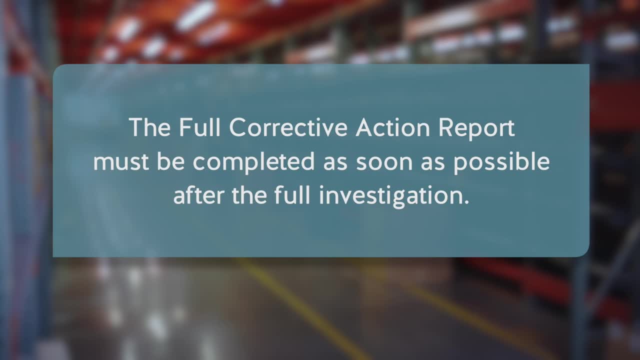 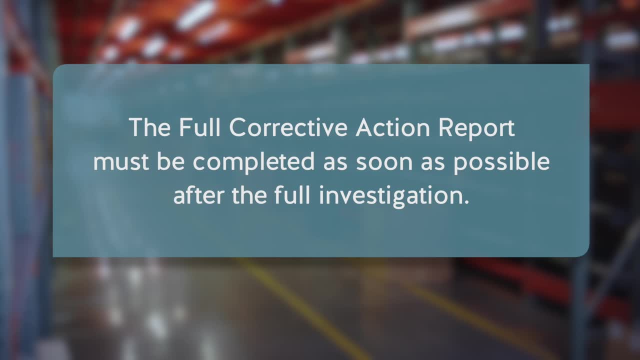 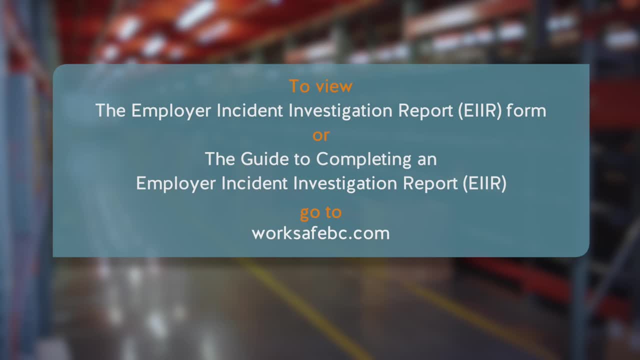 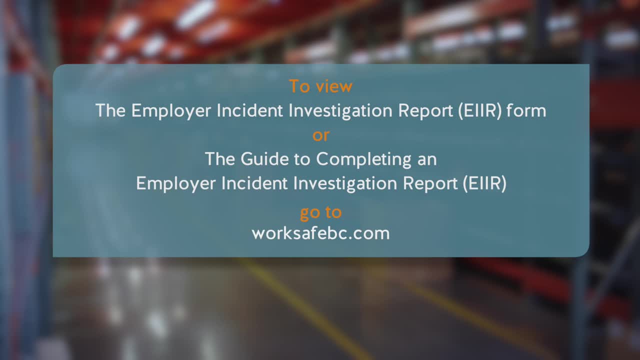 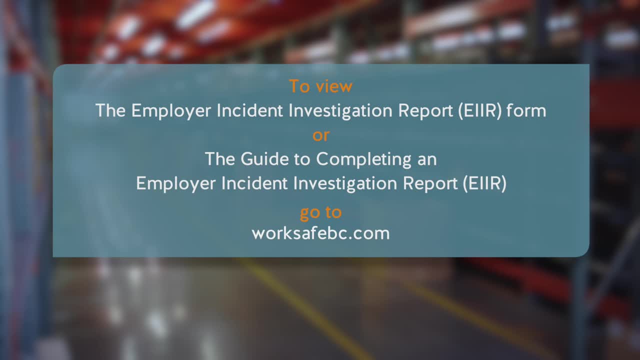 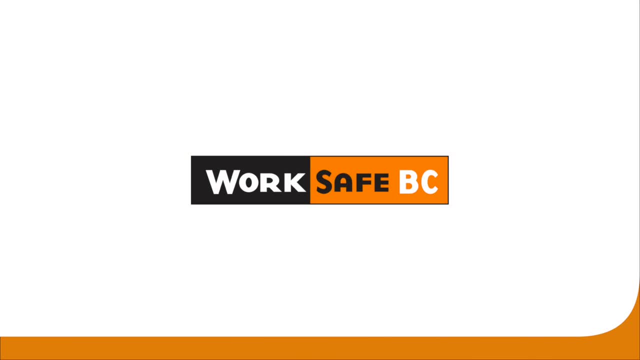 The interim corrective action report must be sent to José González, 02-07-2001.. The interim corrective action report must be sent to dosante. 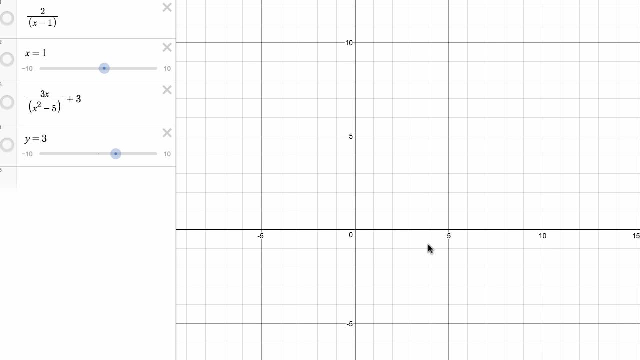 What we're going to do in this video is use the online graphing calculator Desmos, and explore the relationship between vertical and horizontal asymptotes and think about how they relate to what we know about limits. So let's first graph two over x minus one. 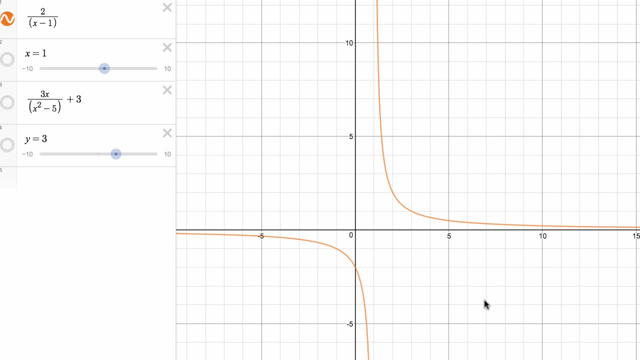 So let me get that one graphed And so you can immediately see that something interesting happens at: x is equal to one. If you were to just substitute x equals one into this expression, you're going to get two over zero, And whenever you get a non-zero thing over zero, 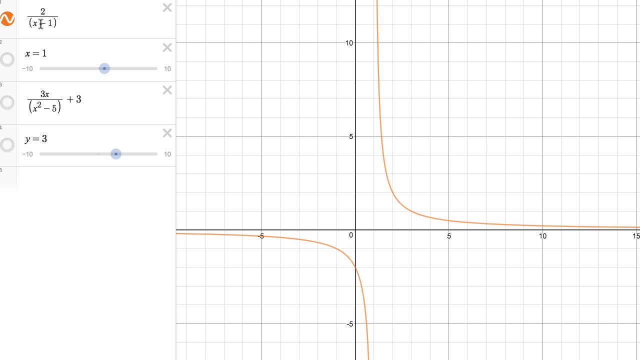 that's a good sign that you might be dealing with a vertical asymptote. In fact, we can draw that vertical asymptote right over here at x equals one. But let's think about how that relates to limits. What if we were to explore the limit as x approaches one?